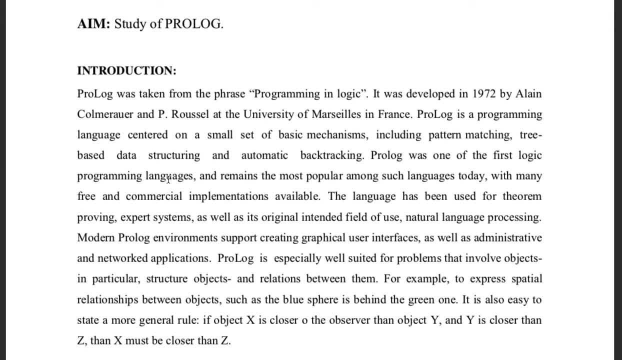 so prologue is used for first logic programming language. so now, uh, what is this first logic programming? so first logic programming is nothing but the predicate logic. now you have to do a little research, read about what is predicate logic, but i'll give you a little hint that, uh, predicate. 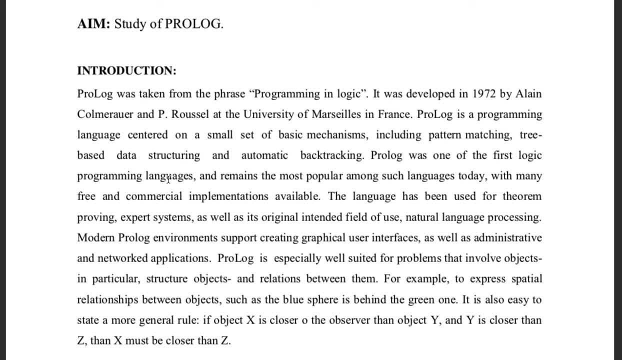 logic is just one step ahead of preposition logic. now, what is the difference? why one step ahead? in preposition logic, you represent, you use connectivities, uh and uh. if the things that are in the connectivity are true, then your whole statement becomes true, right? something like that. 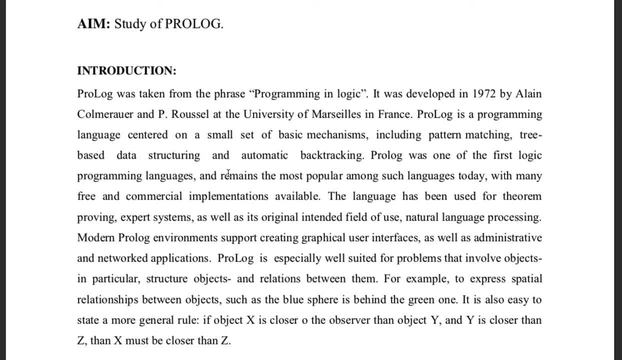 if a or b, then if a is true, then the whole sentence becomes true: a and b. if a is true and b is true, then the sentence is true. this is preposition logic. but now why predicate logic is more powerful, or first, first order logic is more powerful because 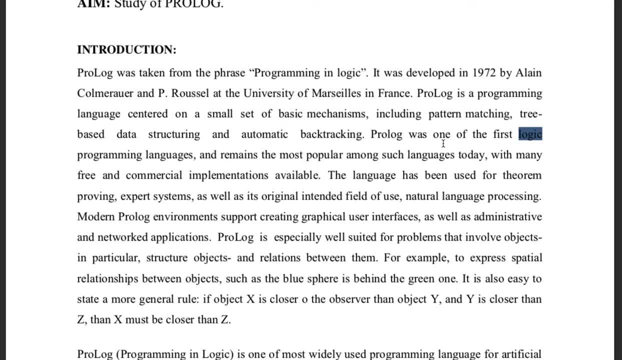 uh, if i say all men are mortal, so then uh, you have to write men and in the brackets you write names of all the men, right? so in this it becomes infinite. very difficult to write in the preposition, but in first order logic you can easily write for all x men. x implies mortal x. 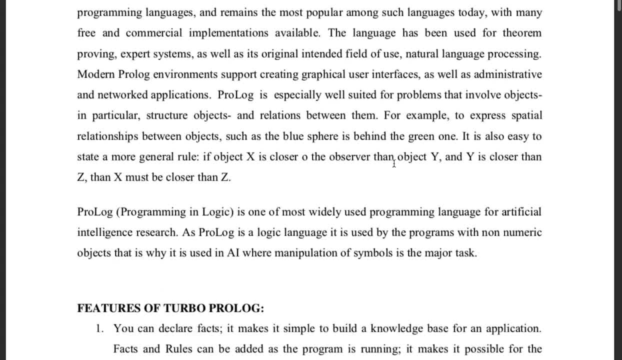 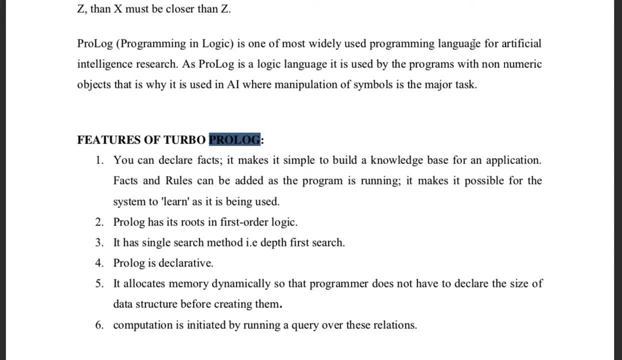 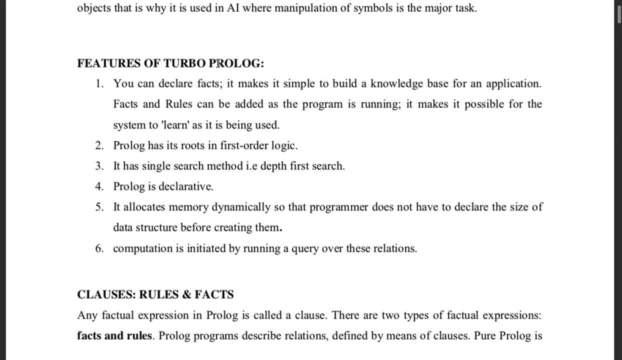 some somewhat like that. you'll have to research it yourself. so features of turbo prologue or simply prologue, as i was saying that, uh, one of the most widely used programming language for artificial intelligence research. that was the main motive why it was developed in the first place. so, features of prologue: it has roots in first order logic. you have to research. 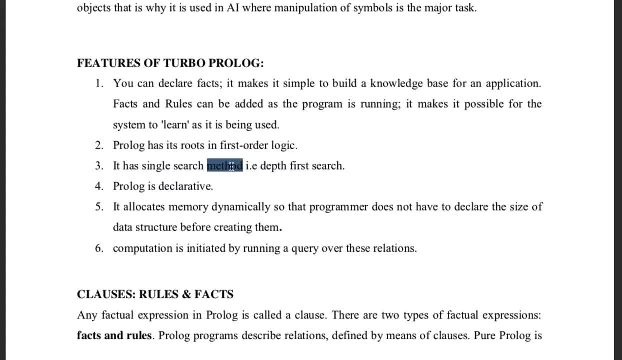 it yourself so as to get a better understanding. so it has single search method, depth first search, and the best thing about prologue is you can declare facts here, so we'll see a little bit more about the facts, but, uh, consider it like you can easily build a knowledge base. 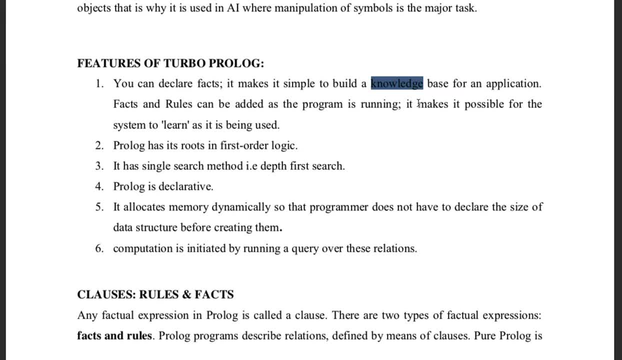 c plus plus is like procedural language in which you have to declare all the rules and all the if i'll statement and switch statement loops before trying to run anything. but in this, to make a simple knowledge base, you have to declare facts and on those facts you can run queries. 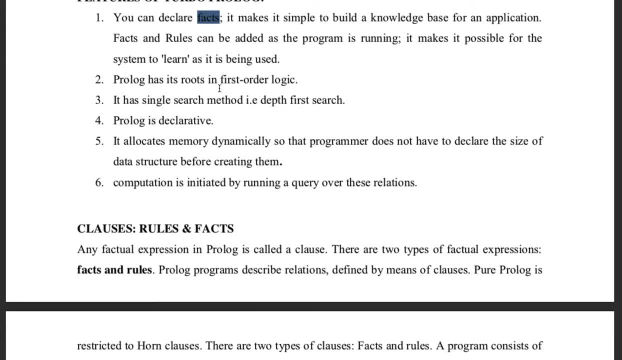 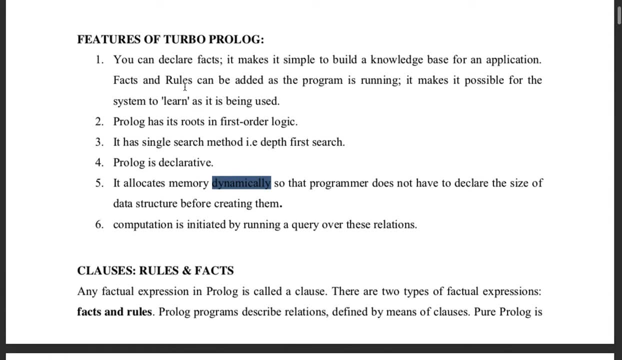 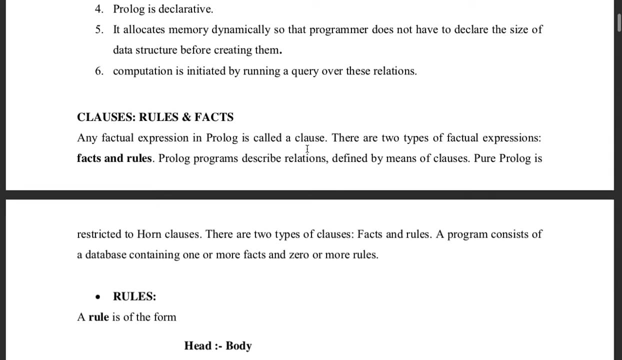 queries mean simple questions, right? so these are the little it has. allocates dynamically memory. so all to say in one is: prologue says you write, you declare things and i'll take care of the rest. so, as i was saying, clauses, rules in fact. so any factual expression in prologue is clause. now what? 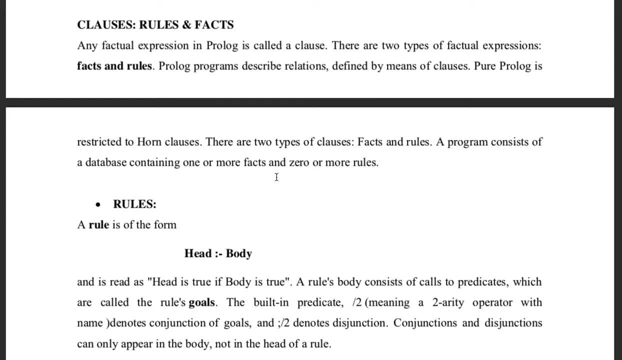 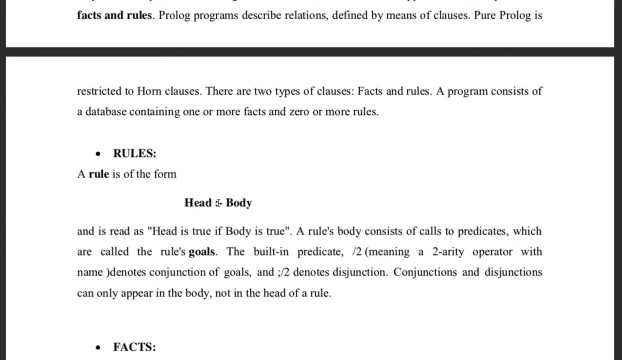 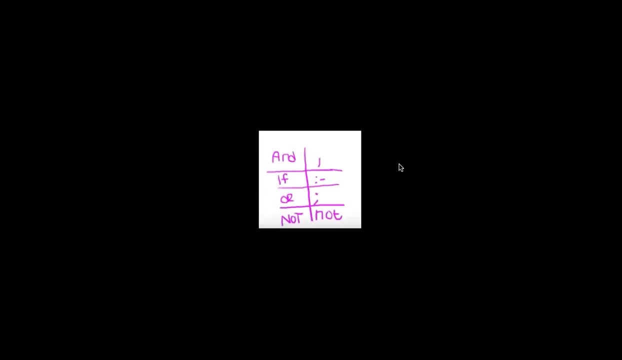 factual expression. there are two type of factual expression: facts and rules. now, rules is of type: this head, something in between symbols and body. now, what is the something in between? i'll show you something, this screenshot i have taken. now, this something i was saying and is shown by a. 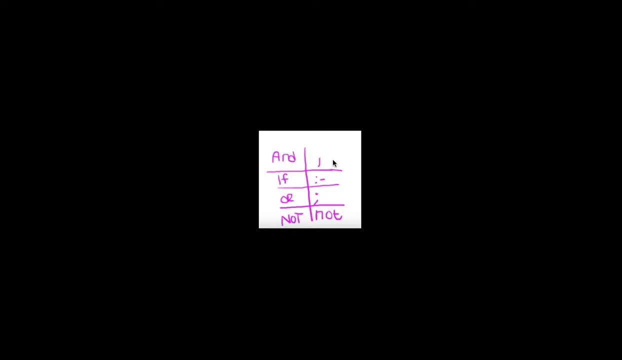 semi, uh, and is shown by a comma- i'm sorry for this, it's a little bit messy, but still- and is shown for comma, if is this symbol messy symbol which i was showing you, and or by semicolon and not by exclamation or by simply writing, not so this was, please remember this- and by comma, if by this colon and dash. so now coming. 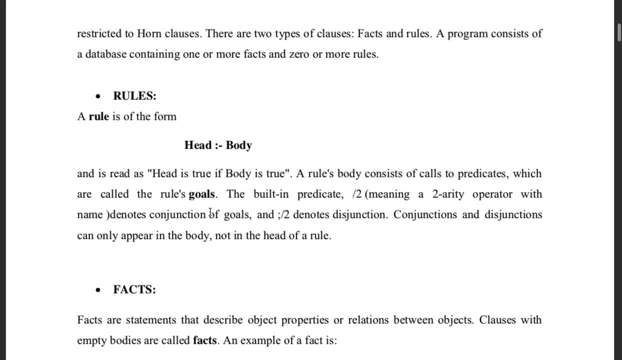 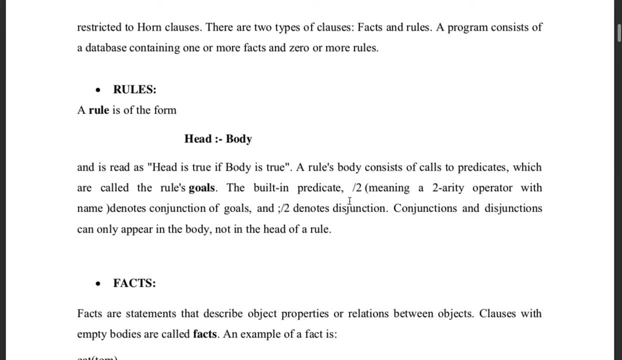 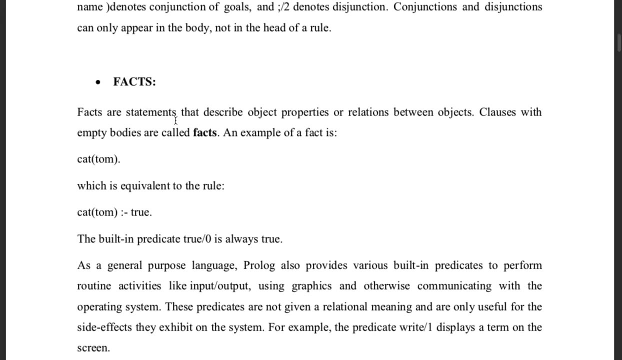 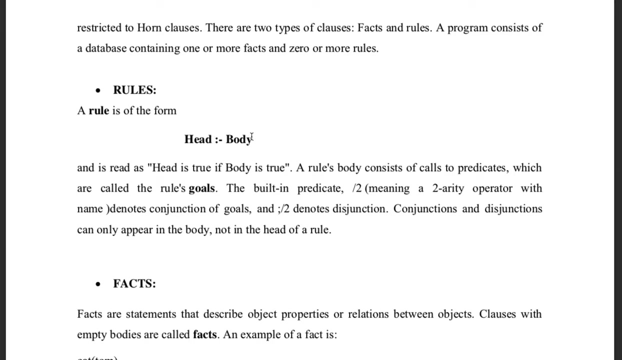 back to the presentation. so it is read: is head is true if body is true? so now we declare rules and those rules are run over facts. so let us first discuss about facts and then we'll see later on. so, as i was saying, that rule is of the form: head, uh, if body. right, this is. 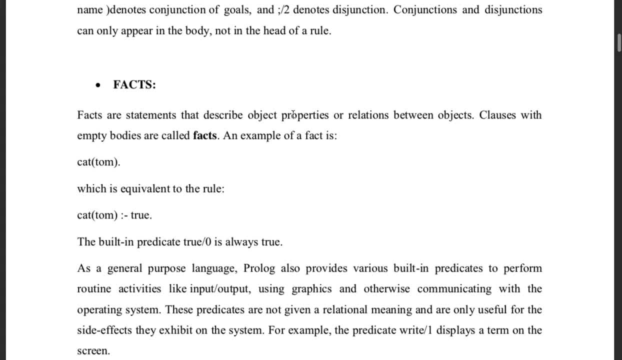 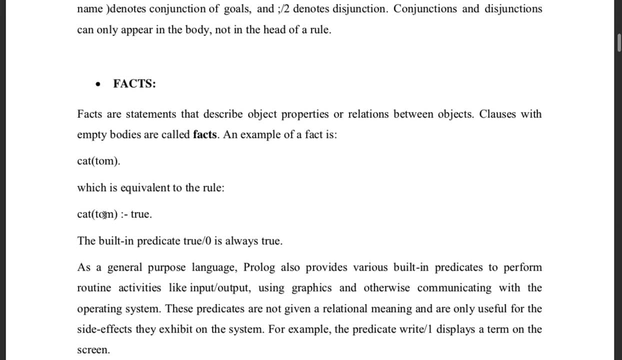 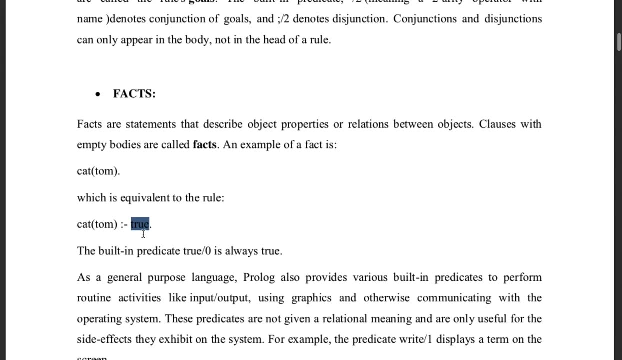 if so, facts are statement that describe object property. so if i try to write fact in that, this form, so it will be like this cat form. if true, so this is head is true. if body is true, body is true, then head is true, right. or you can write fact as this cat term and then dot at the end to end the fact. this is important. 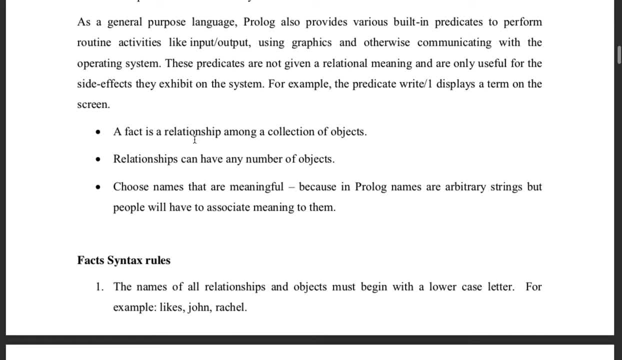 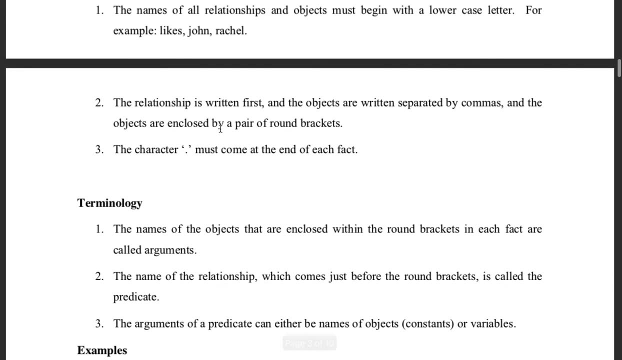 right, you have to write a dot at the end. so facts, what is fact? uh, so in the most intuitive form, i would say fact is a relationship among collection of objects. you show relationship, but the important thing i'll tell you later on. so as we see more facts here, as i was saying, character, 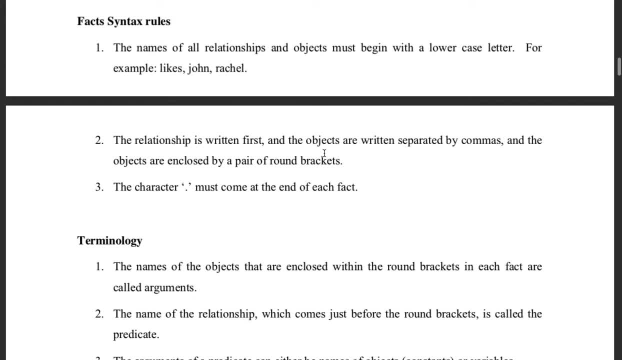 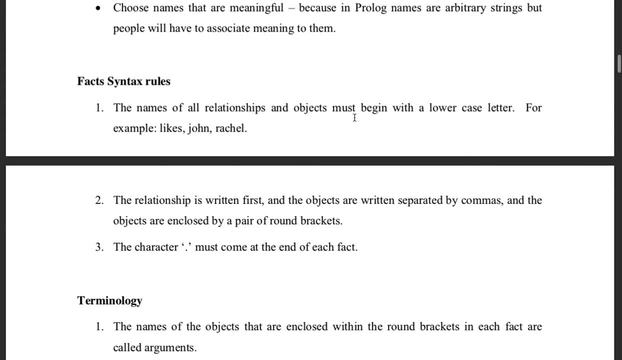 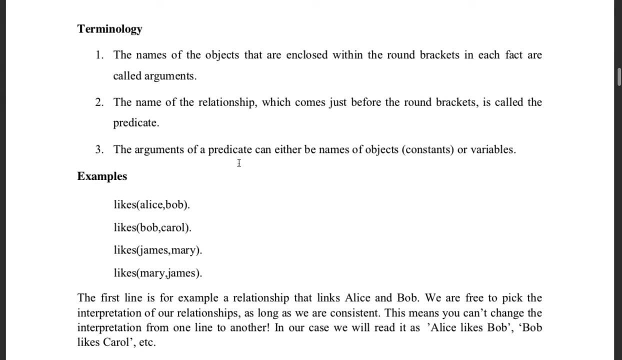 must end. the character dot must come at the end of each fact, the name and relationship. some syntax rule about the fact- you can read it later on- that the name of the relation and objects must begin with the lowercase blah, blah, blah, blah, blah, blah. then terminology. now let us see what we are here. 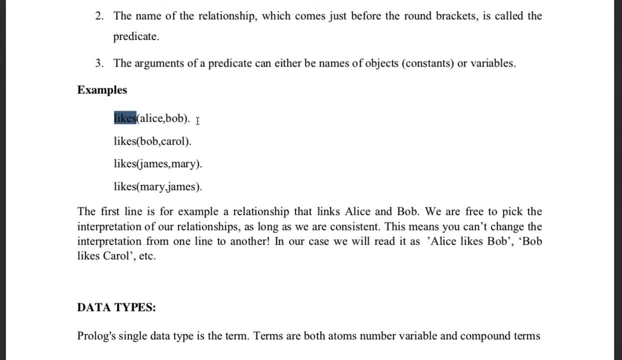 for to learn more, right. so now, if you read this fact, we can see that you can read exactly what happened. so let's go like when i say you can read it anything, anything, anything, whenever you like. fabulous, and the way that i i think we are talking about this. if you write, if you writeaws child, let's say, poi, absolute. 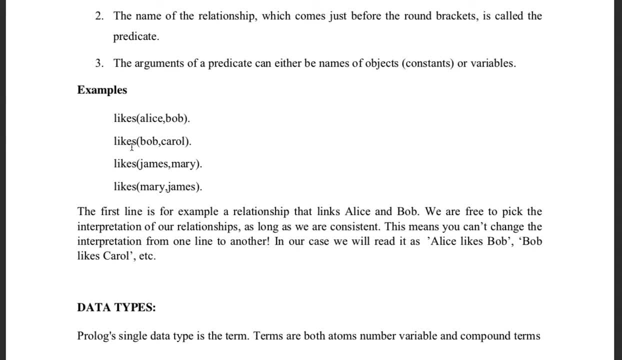 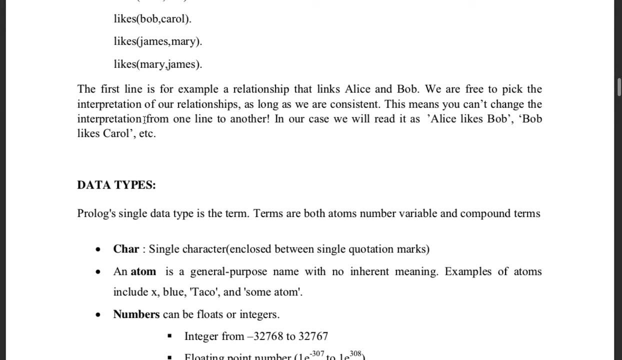 these are the two causes that will cause the нес AK. I have to find what the causes of all that you get. you go back to the life, you go back to the family, you go back to the relationship: bob like carol, james likes mary, mary likes james, not the other way around. okay, that is important. 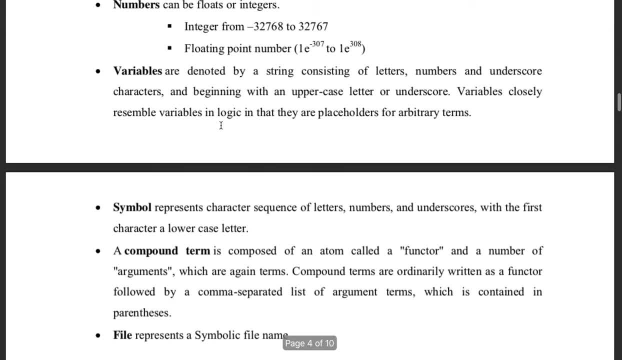 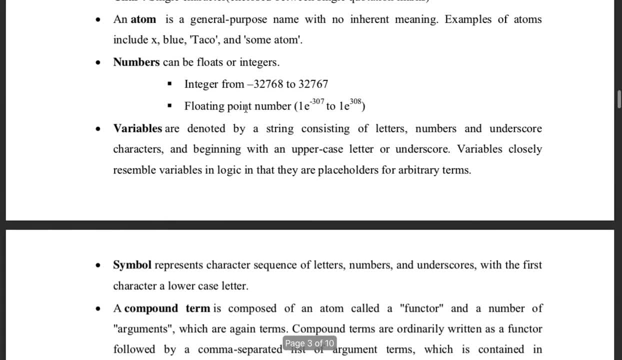 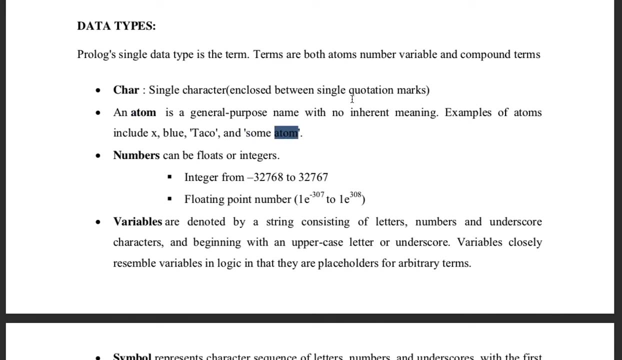 thing. so data types in prologue. um, why, to read this, just come here. these are the various kinds of terms in prologue. uh, so, char. single character inclusions in quotation mark atom- this is also a inclusion. single quotation mark right numbers, variables, symbols, compound terms. you can read. 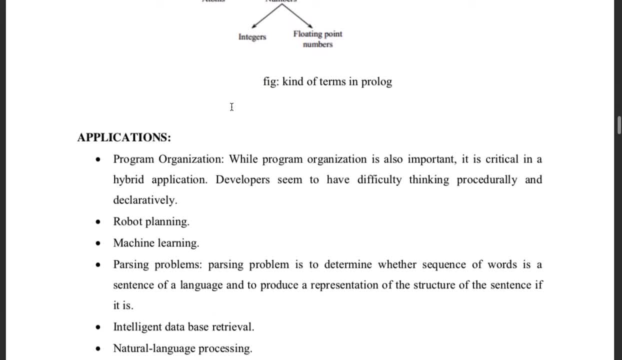 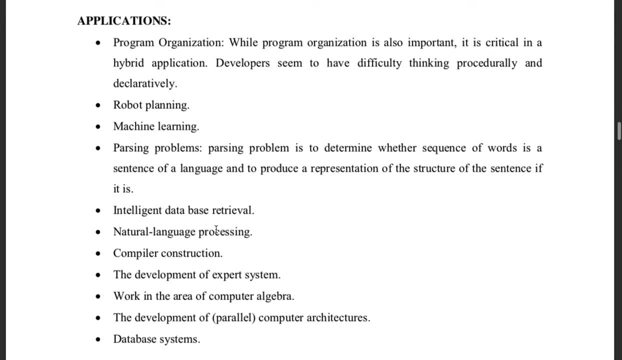 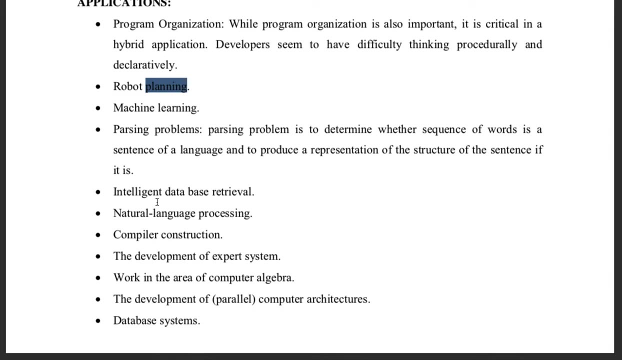 it later on. that is something you can do it on your own now. application: this is, uh, you should know about this because, uh, if anybody asks about what are the application, you must be knowing about it. so it's robot planning, machine learning, ai, i would say, say anything that is related to ai. 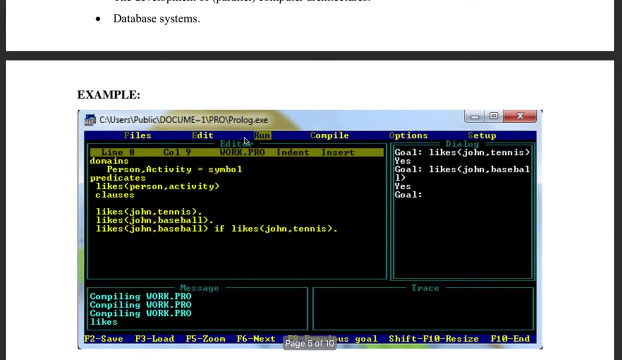 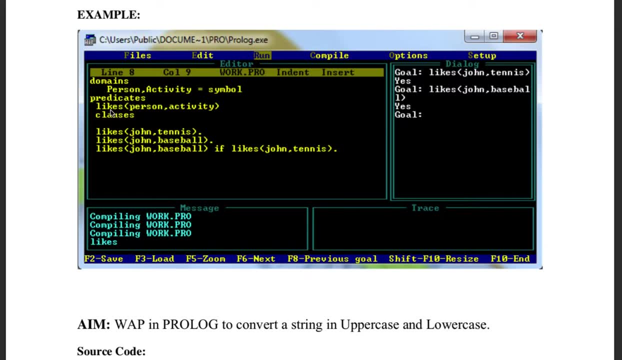 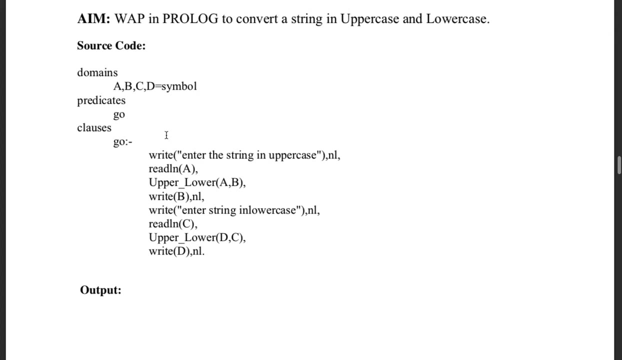 that's something you can say if you don't know anything. a little program at the end. so domains, i would write domains, predicates, predicates. i have explained you. this is, uh, this is like, this is like a fact, right, likes john tennis, likes john baseball. this is my knowledge base. okay, so the program will be seeing, is this a little program?